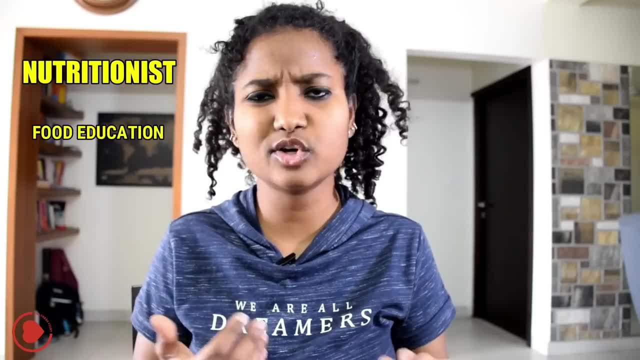 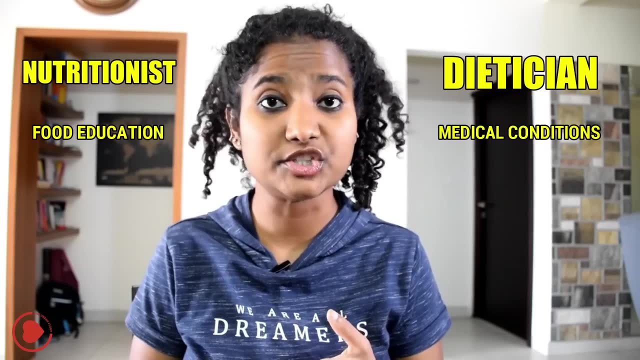 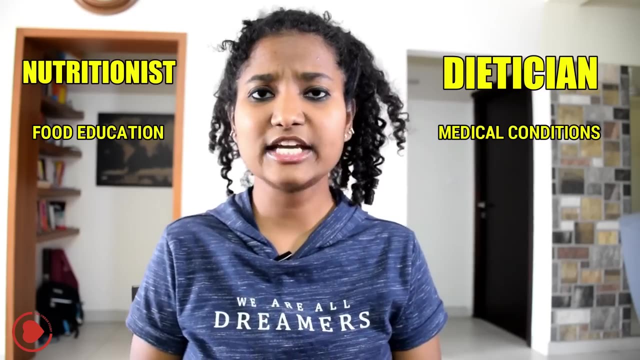 so that they eat better, specifically to increase or decrease their body weight. Dietitians, on the other hand, take care of patients with medical conditions like diabetes, food allergies, cancer, patients recovering from a car accident About what food and supplements to take to recover faster. Think of dietitians as one level above. 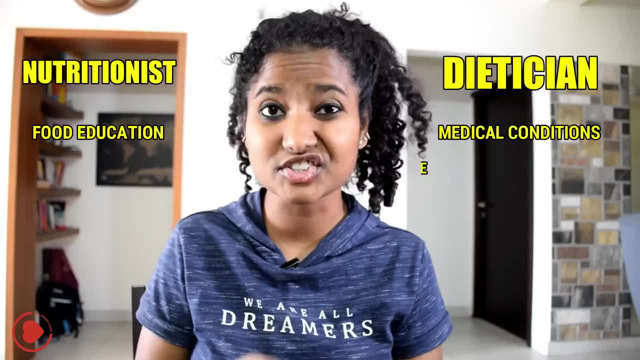 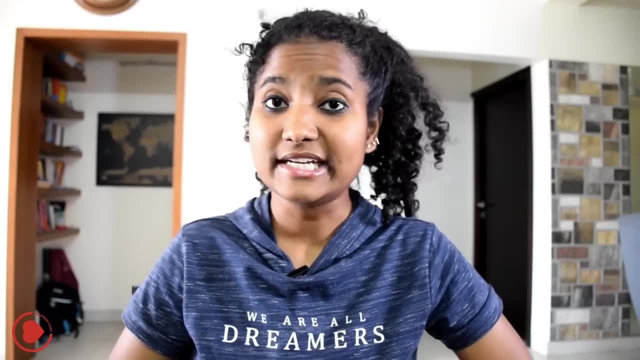 nutritionists because to become a dietitian you need to get a registered dietitian license from the IDA, the Indian Dietetic Association. For example, Ruhita Divekar's website says that she's a nutritionist, not a dietitian. She did her postgraduate in sports science and nutrition. 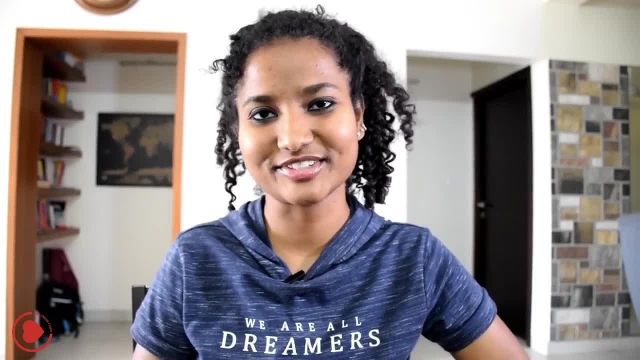 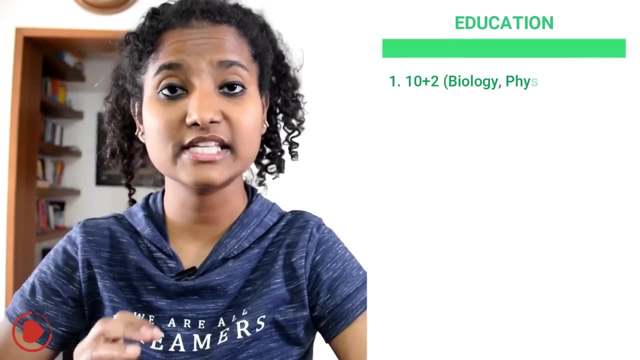 which brings us to what to study: to become a nutritionist. For that you need to pass your 10 plus 2, with biology, physics and chemistry as your subjects. After that, you need to get your bachelor's in nutrition, which is a three-year long course. 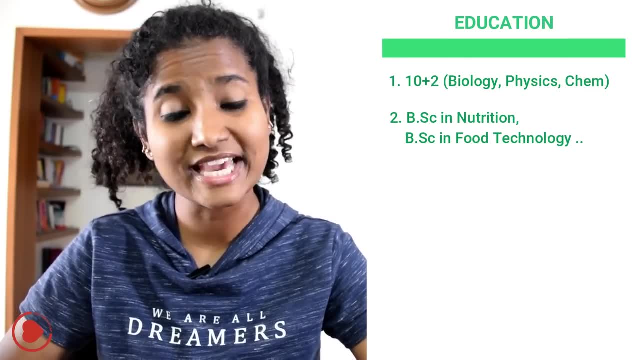 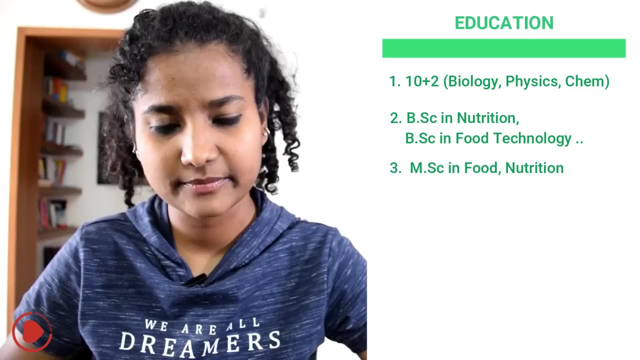 where you focus on basics of nutrition, human physiology, health, weight loss strategies, so on and so forth. Now, after your bachelor's, you can do two things. Number one: get your master's degree, that is, MSc, in food science, nutrition and dietetics, Or you can do PG. 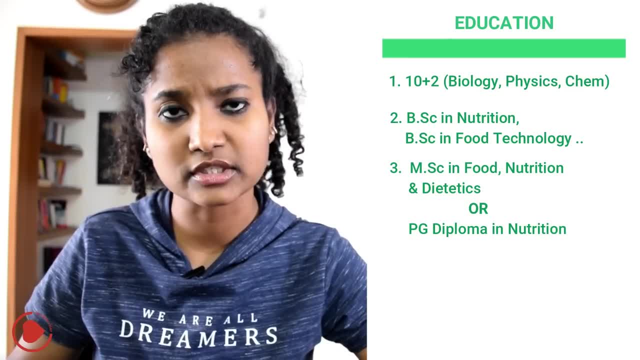 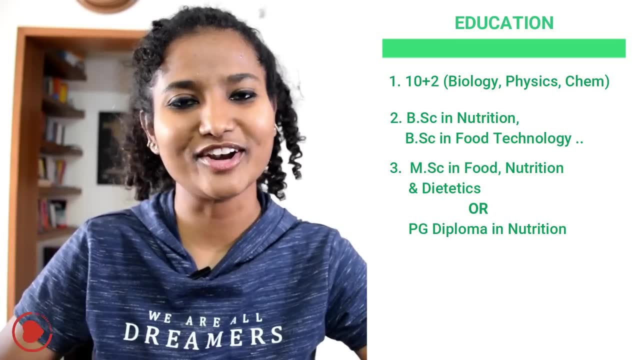 diploma in nutrition, where you can specialize in sports nutrition, public health, pediatric nutrition, so on and so forth, And at the end of your post-graduation or PG diploma, you will be called a nutritionist. Now, if you want to take it to the next level, and 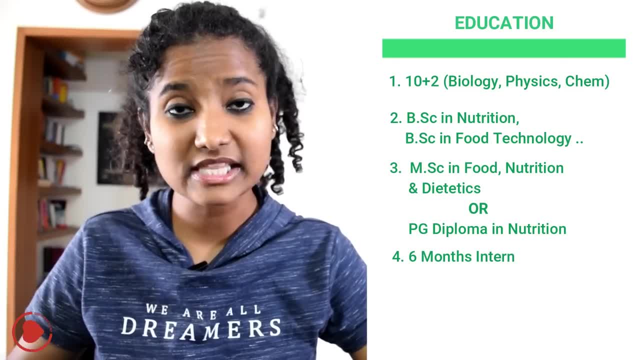 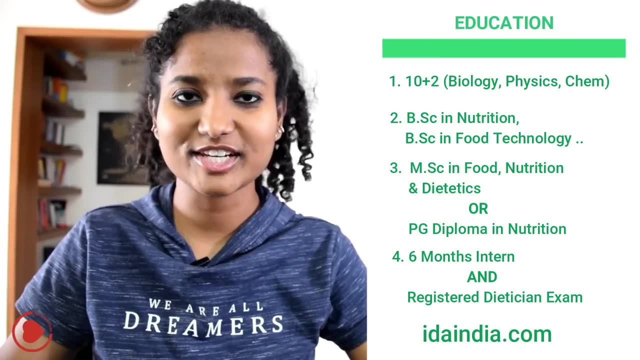 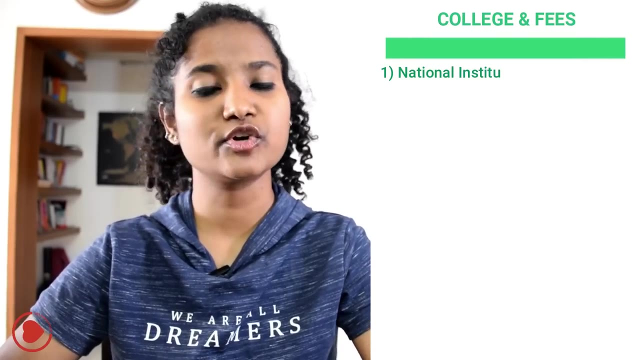 become a dietitian, then you need to intern for six months and write the registered dietitian exam. For more details, check out idaindiacom. I've left the link in the description. You can apply to colleges like National Institute of Nutrition, Hyderabad, SNDT, Women's University. 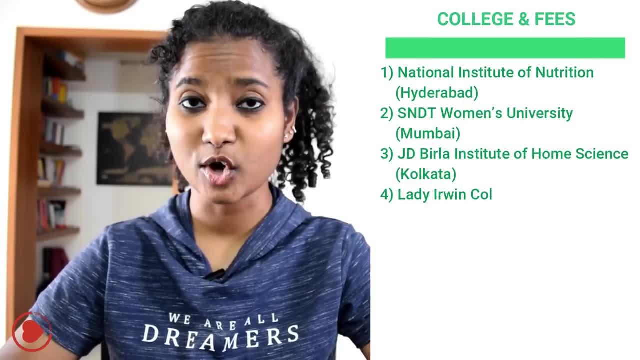 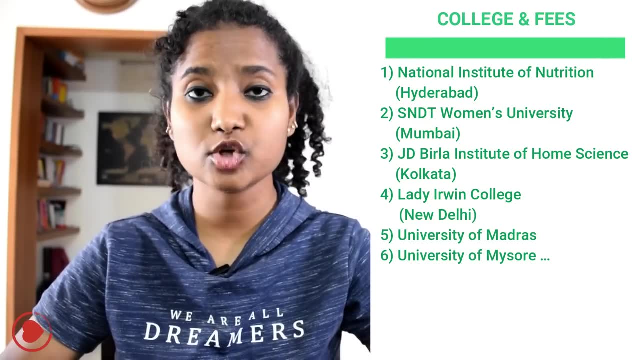 Mumbai, JD Birla Institute of Home Science, Kolkata, lady Irvin College, New Delhi, University of Madras, University of Mysore, so on and so forth. Now, entry into these colleges can be based on merit, or some of these colleges might have their own entrance exams. So make. 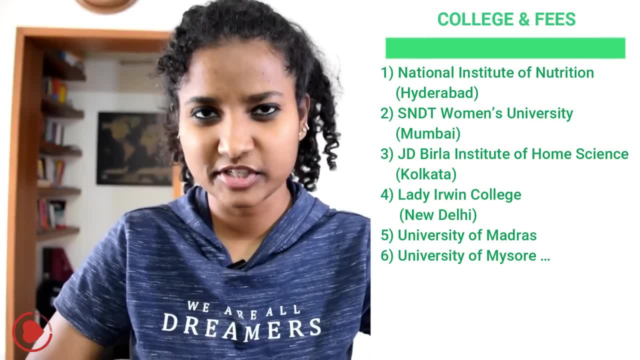 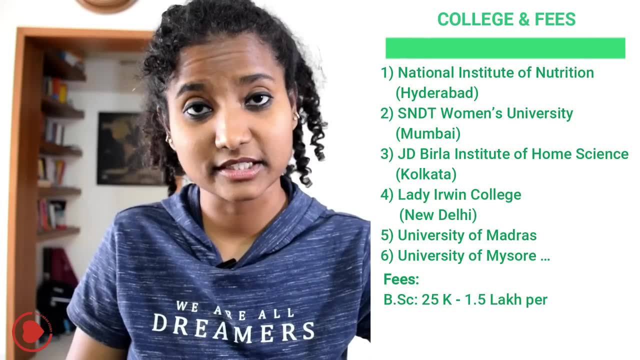 sure you keep checking their websites to know their exam dates. Coming to the fee structure, BSc in nutrition can cost somewhere between Rs 25,000 to Rs 1.5 lakhs per year, And MSc nutrition can cost between Rs 20,000 to Rs 4.2 lakhs. 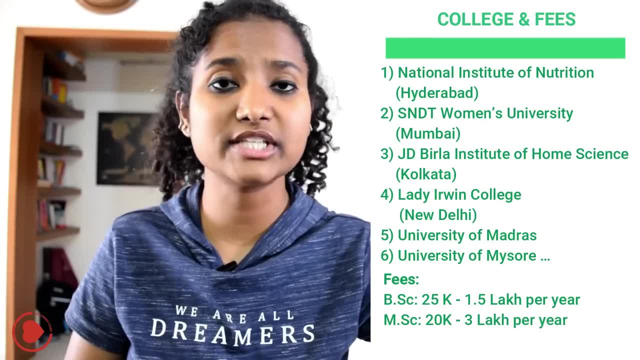 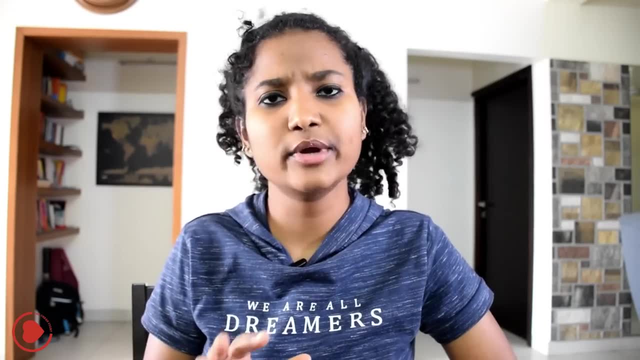 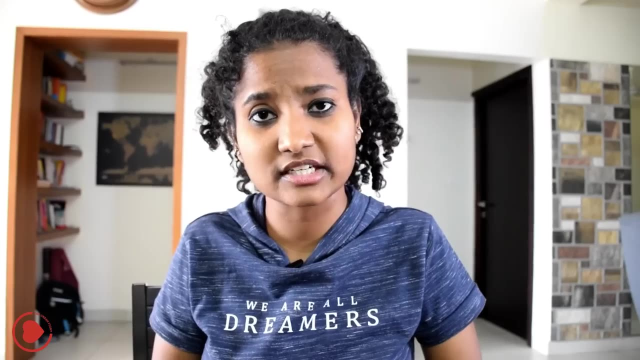 to 3,00,000 per year. It all depends on the college that you get into As a nutritionist or a dietitian. you can work in both government sector or private sector. You can work in R&D, healthcare, teaching and education sector, food products manufacturing. pharmaceutical firms and, of course, fitness centres. You can even be self-employed by starting your own consultancy. Your salary can range anywhere between 10,000 to 50,000 per month or more, depending upon your qualification and your company. And now it's time for the bonus tip. But before that, in case you haven't already, 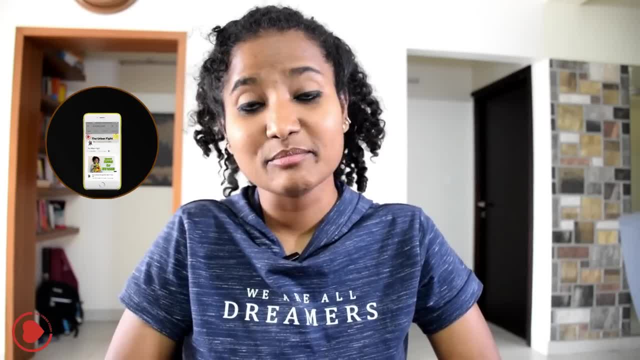 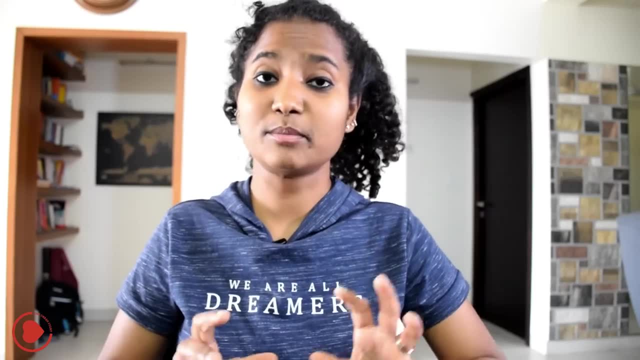 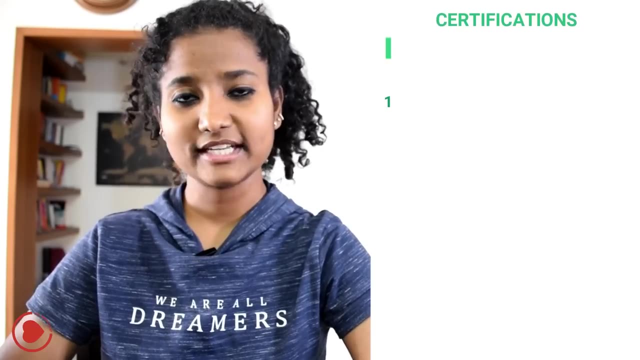 then make sure you subscribe to my channel and hit that bell icon, because I make career and finance videos every week. Now suppose you don't have a science background but want to learn about nutrition. In that case, your options are Number 1.. IGNOO Certification Courses like CFN, CNCC, which are Distance Learning. 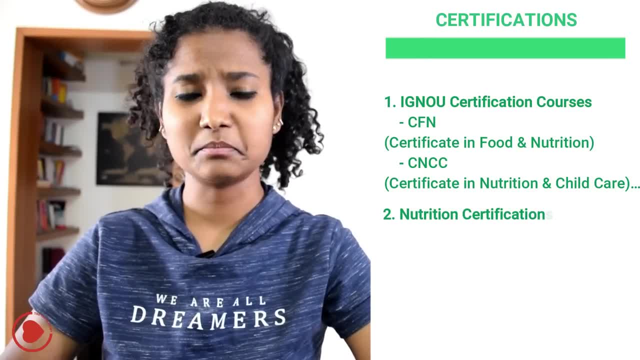 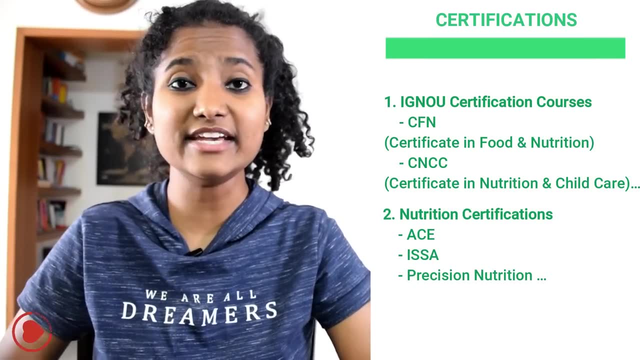 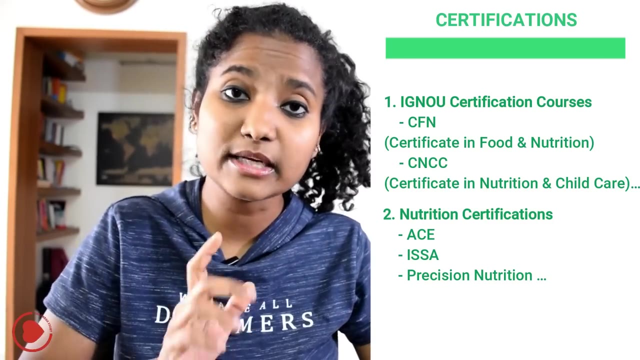 Programmes Number 2. Nutrition Certifications from ACE, ISSA, Precision Nutrition, so on and so forth. Go to their website, read about them and see if that is what you want to do Now. how are these different from a degree? These certifications teach you the fundamentals. 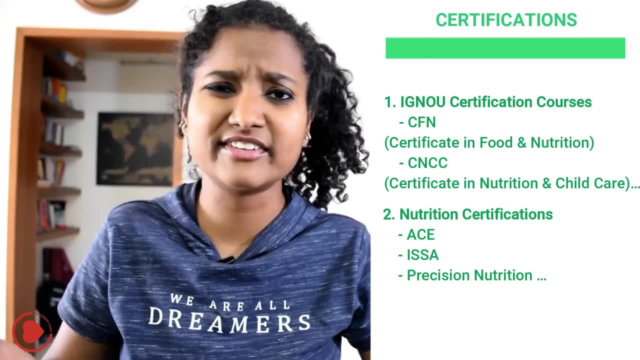 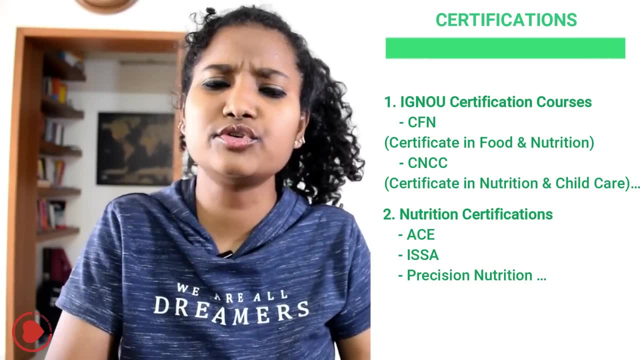 of food intake, about macronutrients, micronutrients, body weight, so on and so forth, which come in handy if you're already a certified fitness expert and want to offer nutrition lessons resources to your clients. But you cannot prescribe, diagnose or cure a patient. 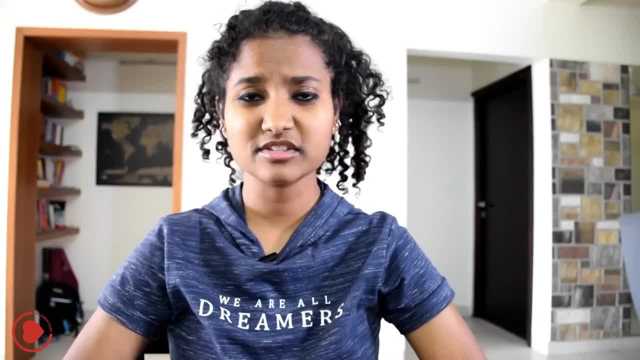 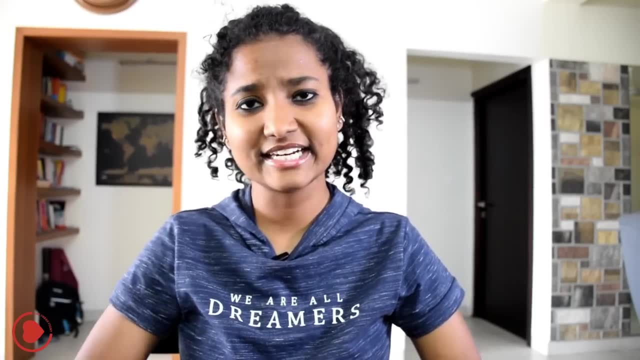 See, India is becoming health-conscious these days, which is why all these people are jumping in and providing fat-cutter drinks and fat diets, just to improve their click rate and make a quick buck. But what will set you apart from these clowns is 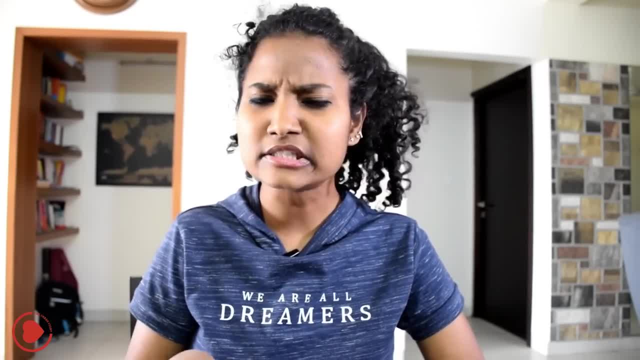 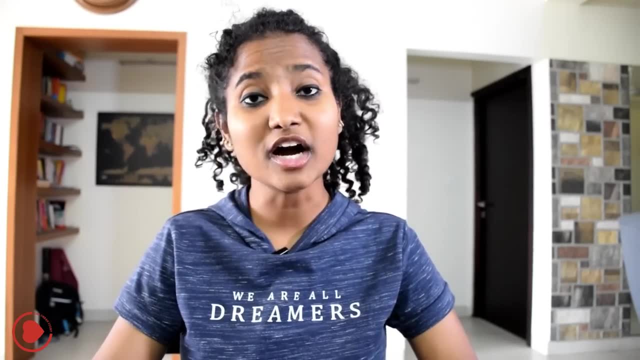 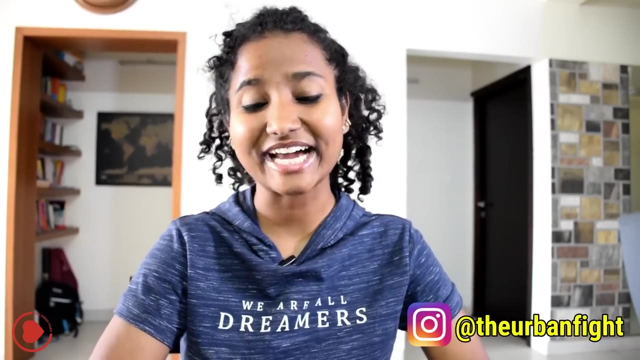 Proper knowledge and experience, which only a certified dietitian or a certified nutritionist will have. It might take time to get there, but in the long run, integrity always wins For more such Gyan. follow me on Instagram, because that is where I ask you which video you want next. 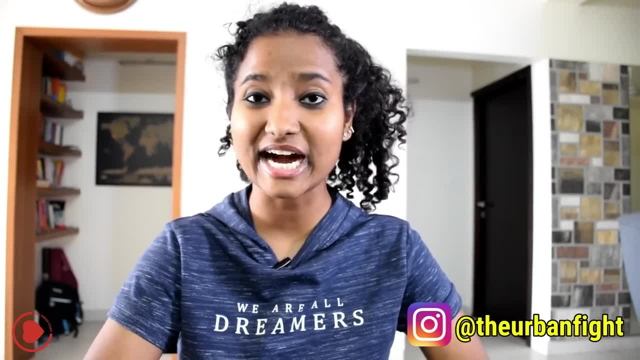 On that note, I promise to see you again next week. Until then, keep fighting the urban fight to be fit.